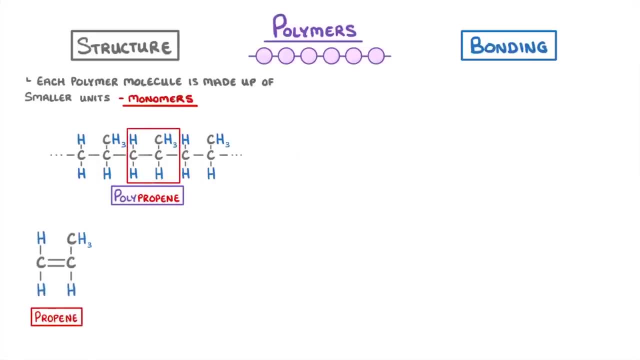 made from these monomers called propene, which have the formula C3H6. And if we line a few of them up, you can see how they could keep adding together again and again until they form a huge polymer chain. Now the important thing to be able to do is notice that a particular molecule could. 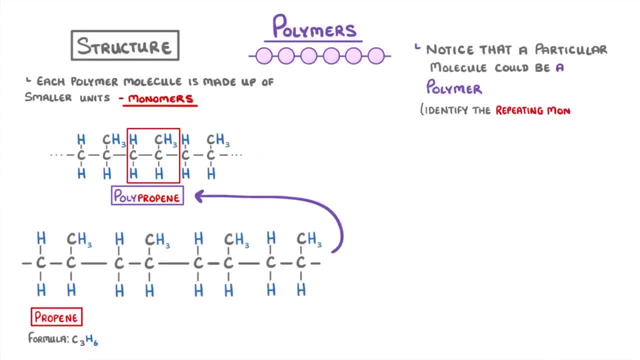 be a polymer and identify the repeating monomer. For example, we can tell that this polypropene we just made could be a polymer because we can pick out a small section that seems to repeat. Then, once we've identified this repeating unit, we can draw it out by itself And you'll. 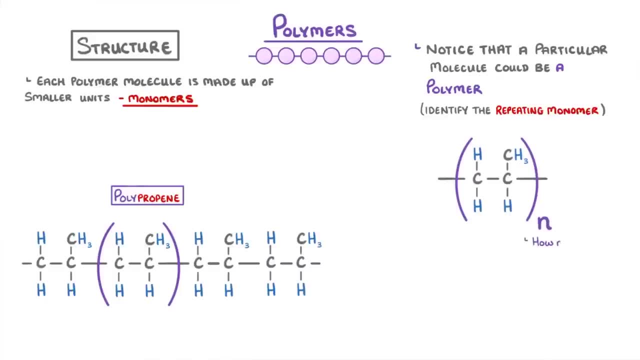 often see the letter N in the bottom right corner, which represents how many of those repeating units there are. So if we wanted to write a reaction for combining 400 propene monomers, then instead of drawing out the entire polymer as a product, which would take us ages, we could just draw the 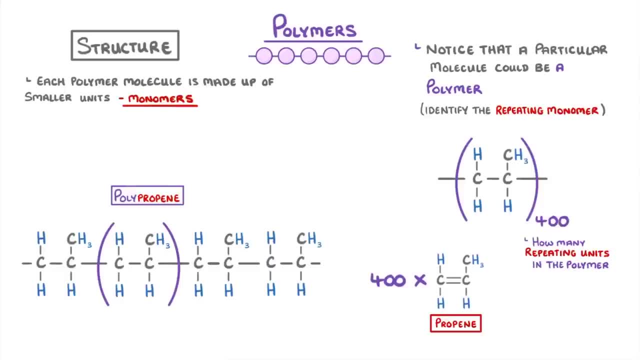 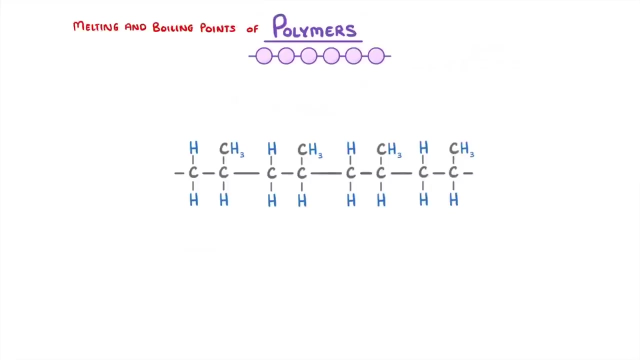 repeating unit and put 400 in the corner. In general, though, we just put N instead of actual numbers. The other thing to notice with these repeating units is that we always use curved brackets and we show the bonds coming through. Now the last thing we need to look at is the melting and boiling points of polymers. 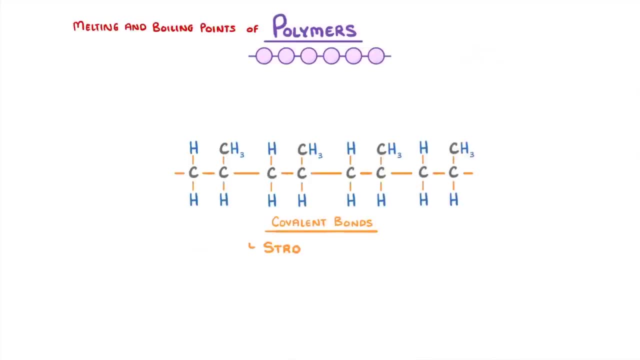 The bonds within the polymers are all covalent bonds, which are really strong and so would require really high temperatures to break. However, to melt or boil polymers, it's not actually these covalent bonds that we need to break. Instead it's the intermolecular. 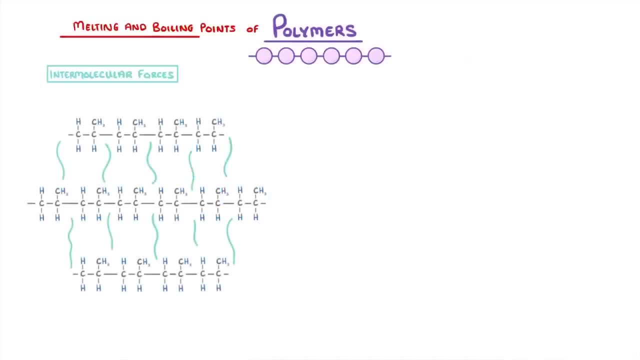 forces between the separate polymer molecules. These intermolecular forces are the ones that break the bonds that are covalent and these are the intermolecular forces between the separate polymer molecules. And these intermolecular forces are much weaker than covalent or ionic bonds. 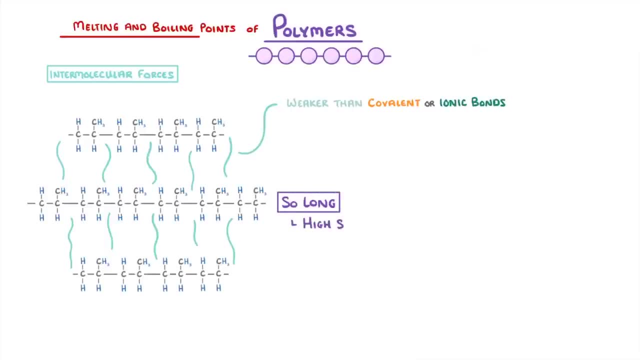 However, because the polymers are so long, they have a high surface area, and so there are loads of these intermolecular forces, which means that to break them all would still require quite a lot of energy. So, although polymers have lower melting and boiling points than giant covalent structures,